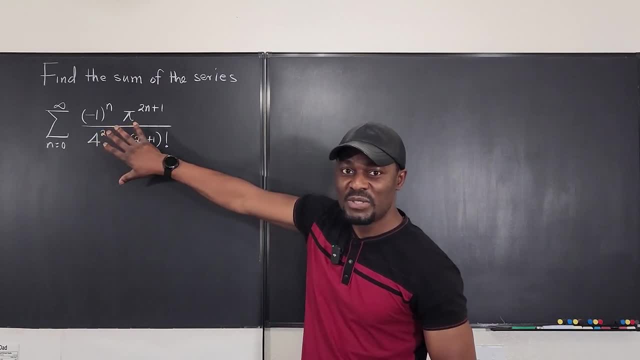 because you're given the Taylor series representation of a particular function and you have to be able to see that. So whenever you get a formula like this and you're asked to find the sum of the series, it's because you're expected to recall some of the standard series. 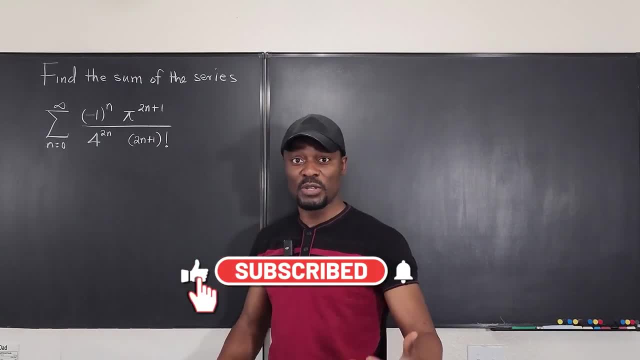 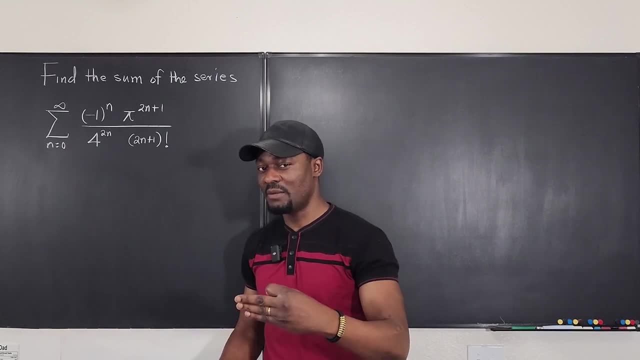 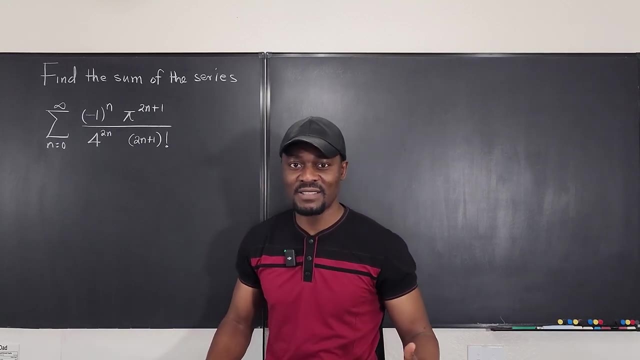 Taylor series expression for some popular functions, And the most popular ones are e to the x, sine of x, cosine x. So you might throw in maybe 1 over 1 minus x, or they might throw in arctan x. You have. 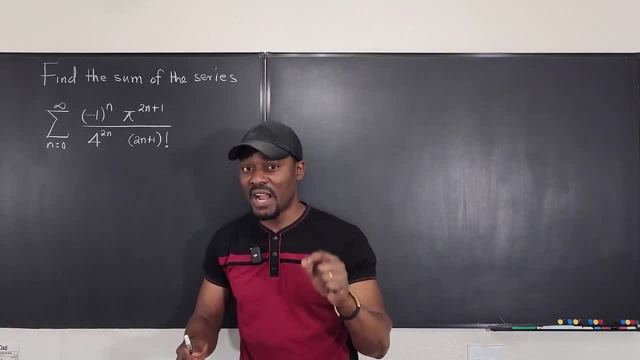 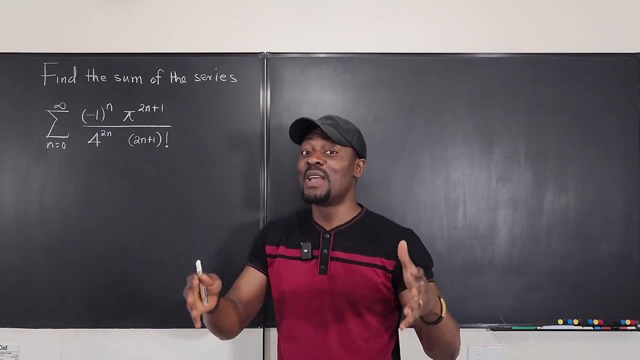 to be able to know what those characteristic functions are, as a calculus 2 student or whatever level of calculus you're taking. So it's required that you know what the sum, the Taylor series representation, is for each of these three functions. I'm going to write, So the first, 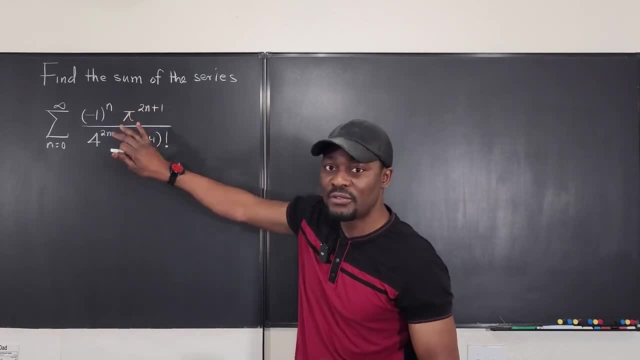 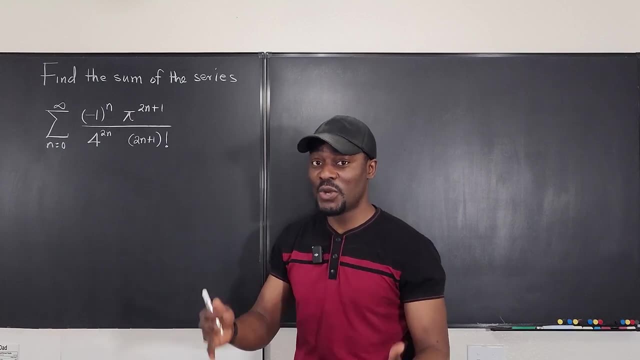 one is e to the x. You're going to compare whatever you have to e to the x, if it looks like it. If it doesn't look like it, it's not it. Then you move on to sine x, then you move on to. 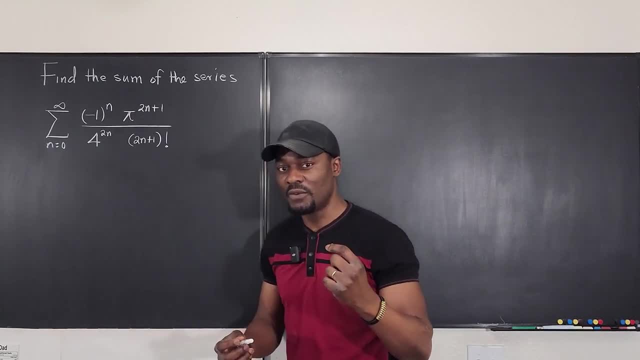 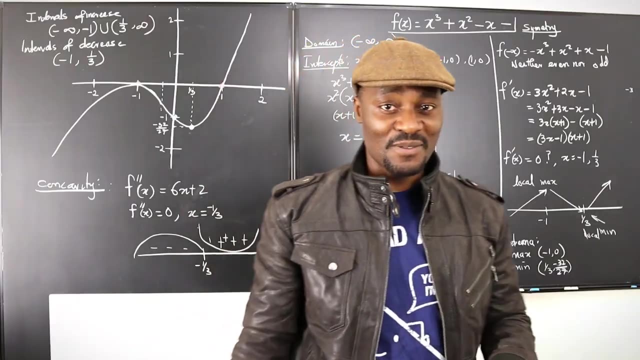 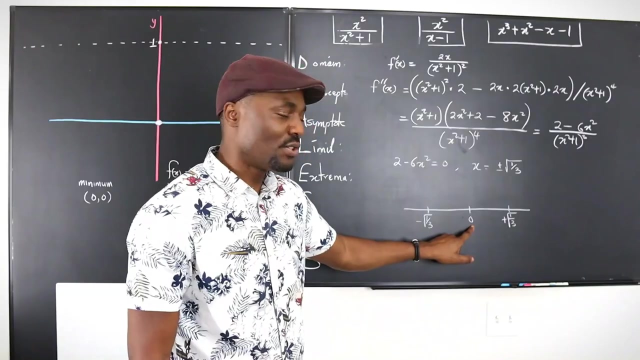 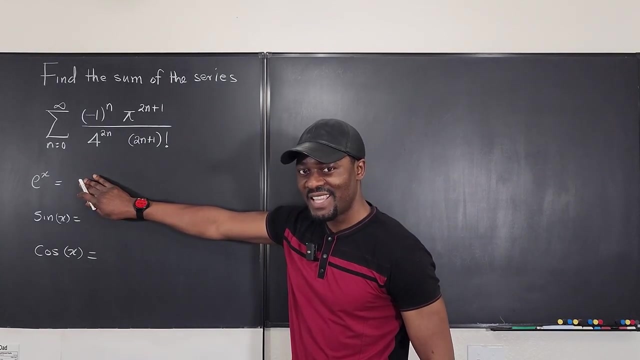 cosine x. So what is the Taylor series representation for these three things I just mentioned? Let's get into the video. The representation for e to the x is the simplest And which you must know. okay, You can't say oh, I forgot or I mixed it up, It has. 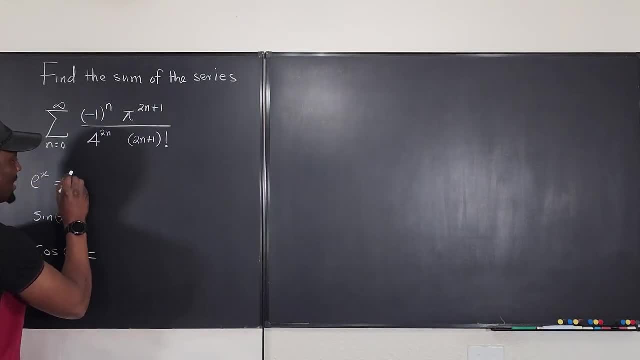 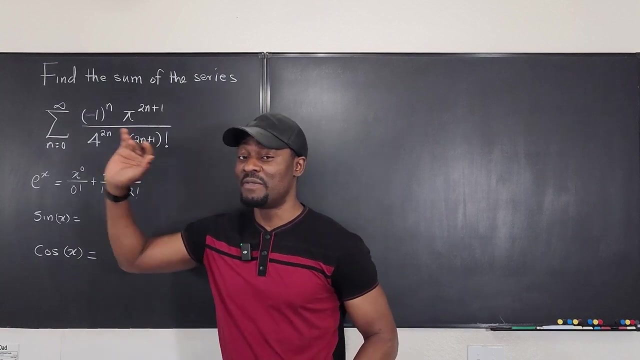 to be. the easiest way is to write it this way: It's x to the zero over zero factorial, plus x to the one over one factorial, plus x to the two to the second over two factorial. You see how this one does not require any memorization. You're going from zero to infinity. 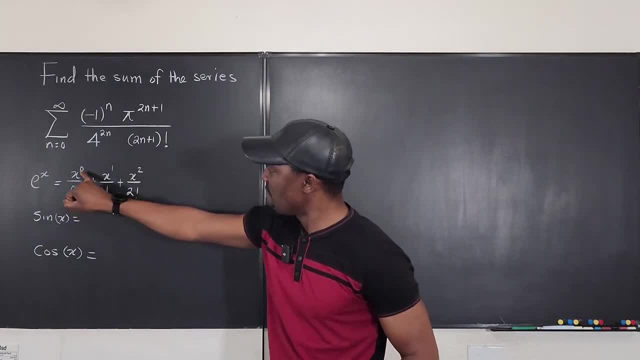 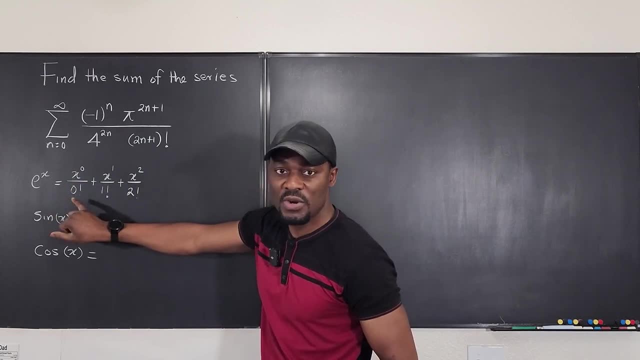 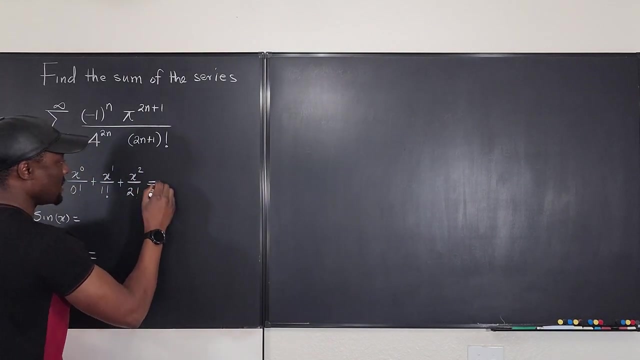 That's it. You start from this, but we can evaluate the first one. Anything to the zero power. as long as x is not zero is going to be one and zero factorial is one. So the first term here is one. So in some expressions this could be written as one plus and the 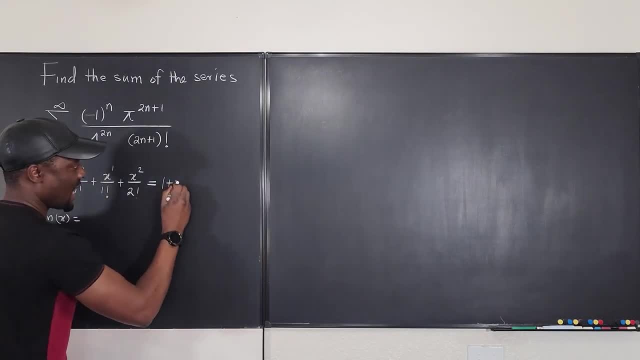 next term is going to be x to the one over one factorial, which is x plus, and you keep going: This is going to be x squared. So in general, you usually have it written this way. Okay, It goes on, but there's a short formula for it. This is the same, So this: 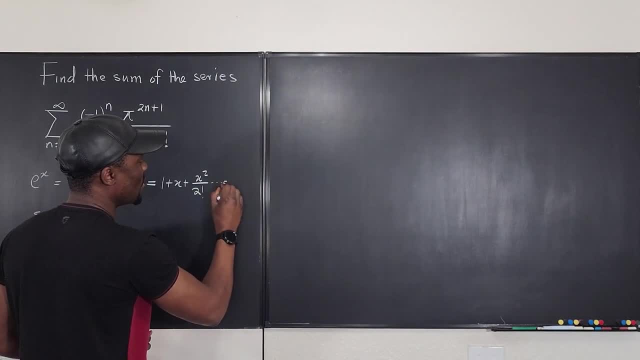 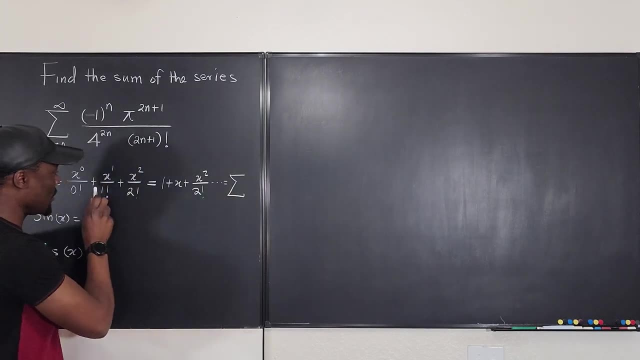 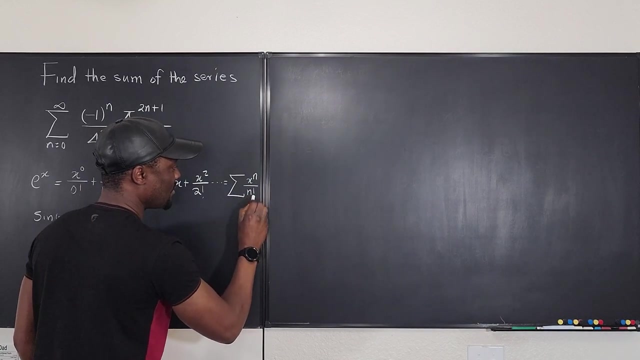 keeps going until you just say: okay, the total of this is the sum. I'm not going to do that for this one. I'm just going to write this final formula. This is from what you see. it's basically x raised to power, n divided by n- factorial. That's it. That is an easy. 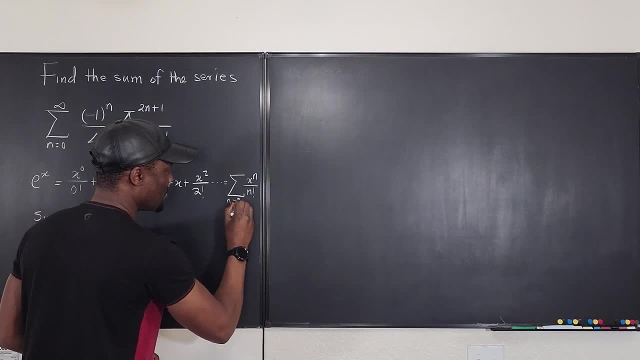 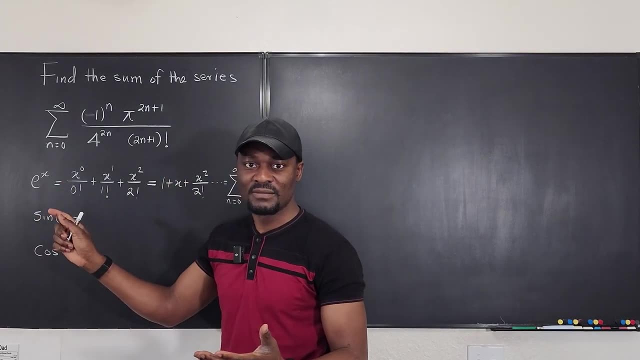 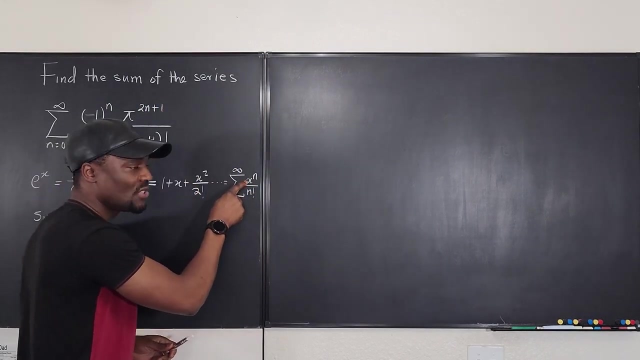 way for you to write this. So we say n goes from zero to infinity, Zero to infinity. This is the Taylor series representation of e to the x. So if you get a problem where in the formula given like this, what you see here is not x, If they 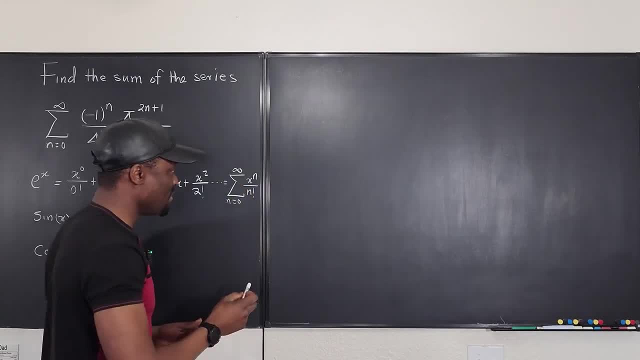 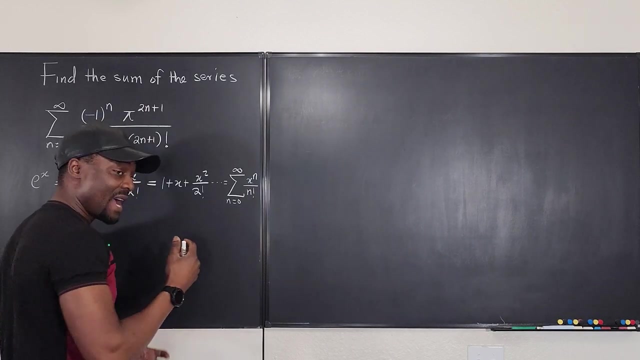 put the number two there. okay, then it means you just need to replace x with two, So e squared can be written in short form as two to the n over n- factorial, And that's it. So it's the same idea you're going to apply when you're dealing with sign of X. So what? 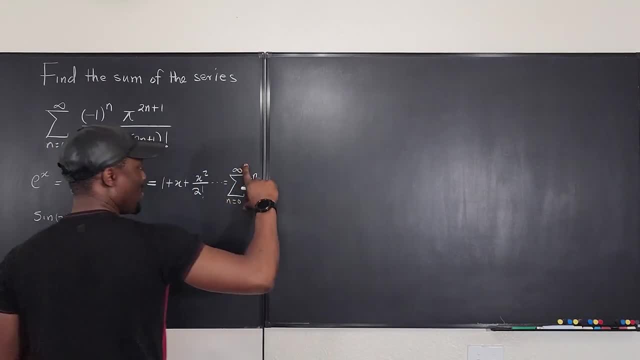 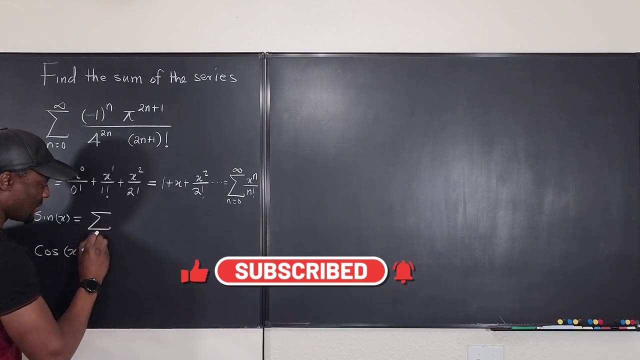 is the Taylor series representation of sign of X. I'm just going to write this kind of formula, which is going to be equal to the sum from n equals zero to infinity, of negative one raised to power and multiplied by. Since this is X, it's going to be x raised to to. 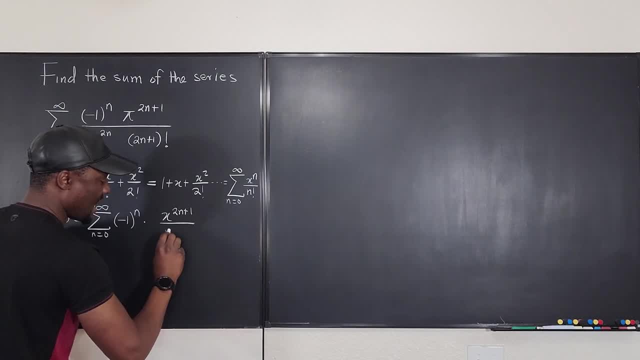 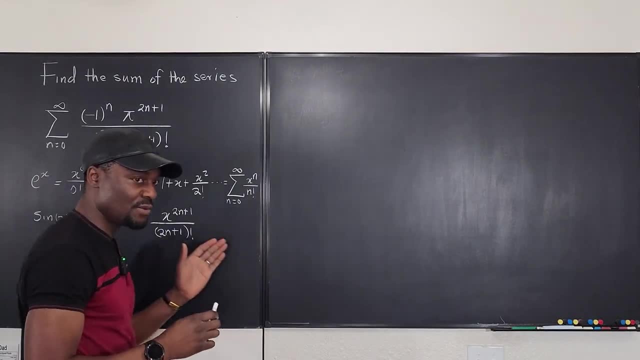 n plus one plus x squared, And this is the whole formula. So I'm just bringing in the sum, the sum in 2021.. This would be equal to the sum of negative one to infinity, of divided by n to n plus 1 factorial. this is the Taylor series representation of 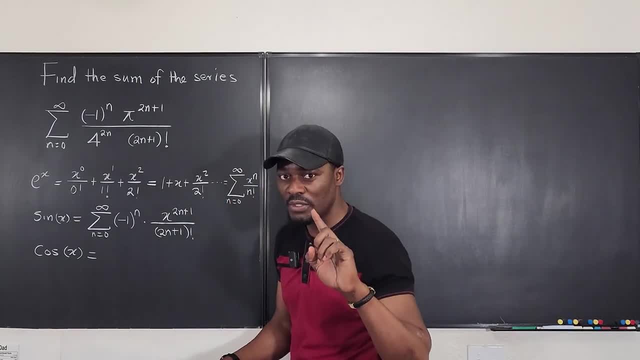 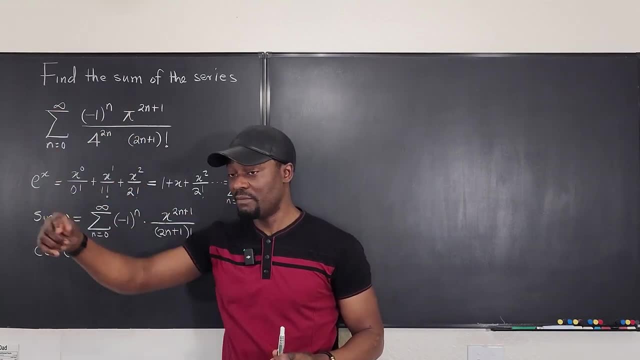 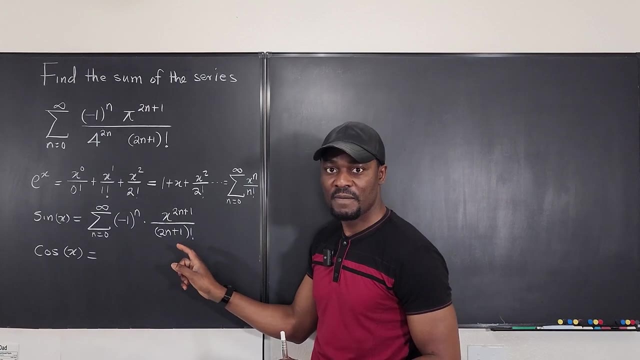 sine X. remember it's important to know there's always a negative 1 raised to power n, because for trig functions they fluctuate, sine and cosine. they fluctuate between positive and negative, and that's why this is there. otherwise, this should be your focus now. what would happen if it was cosine? well, is this. it's very. 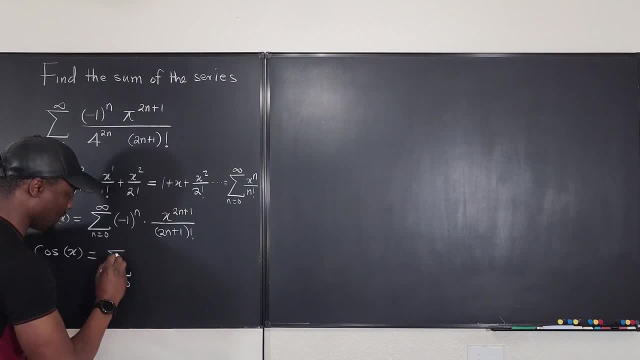 similar to it. it is a sum from n equals 0 to infinity, of negative 1 to the n. multiplied by this is now going to be X to the just 2n over. this is going to be just 2n factorial. you have to recognize the difference between this and this and 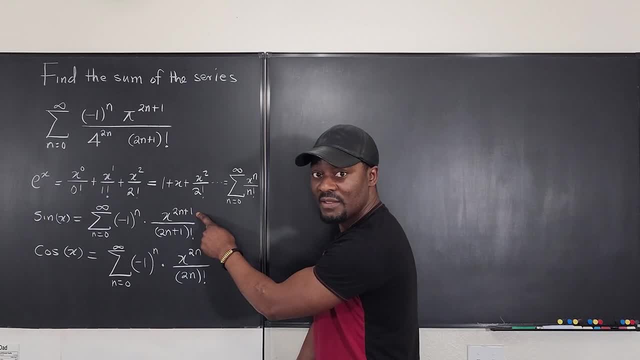 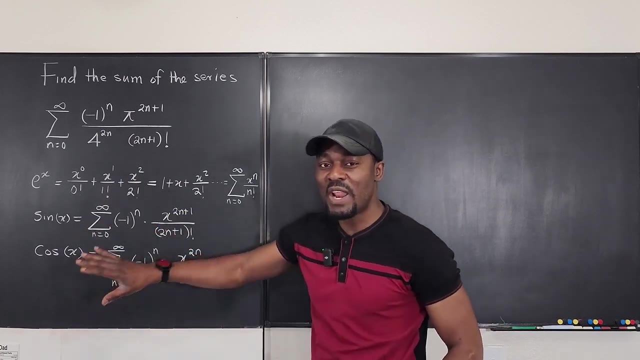 look at the difference is just this one. remember that when you integrate cosine X, you get sine X, and when you differentiate this, you get this. that's it, ok. please remember these three so that whatever problem you get on your test or whatever you're doing, you can answer the question. so now let's go to this. 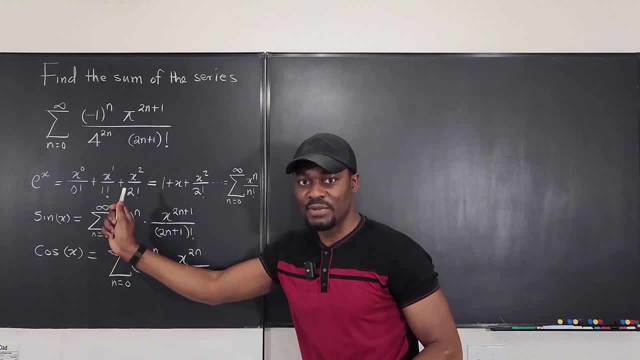 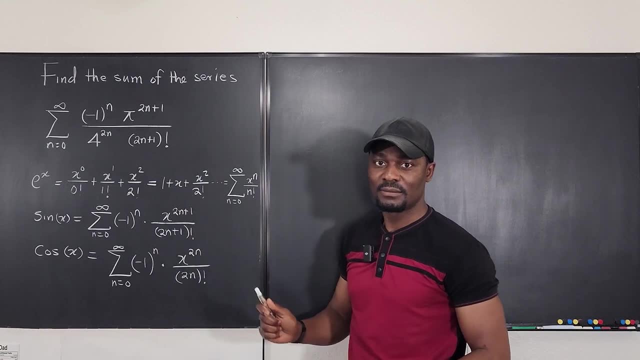 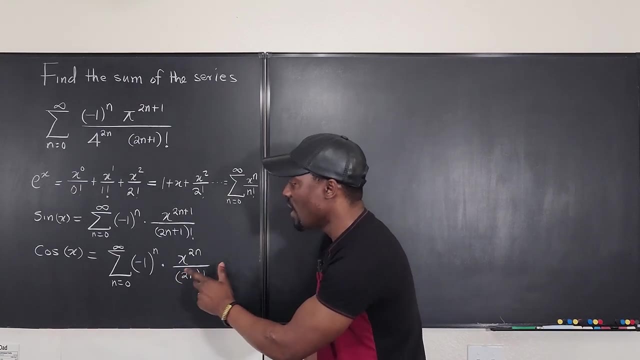 question what? which of these functions? because we just let's, just because I know the answer is one of these. which of these functions looks like this: clearly it is the sine function. just because you look at the factorial. now, the factorial may be difficult to manipulate. the exponent is: 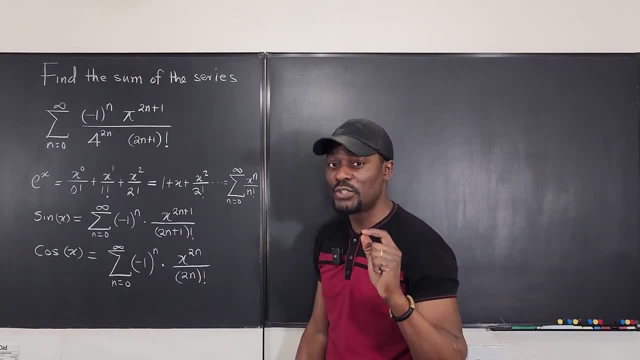 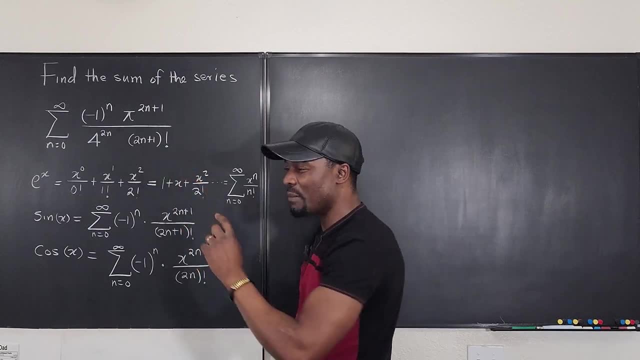 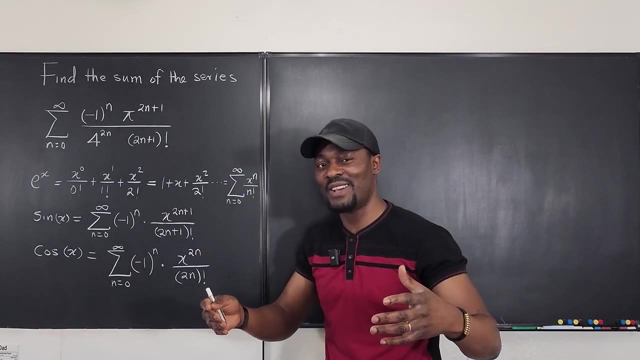 easy to manipulate, but the factorial might be difficult. so what you want to focus on is the factorial. so I look at this. I see that this factorial looks just like this, so I'm going to assume that whatever I've written here is the sign of something. I just need to know what that something is. 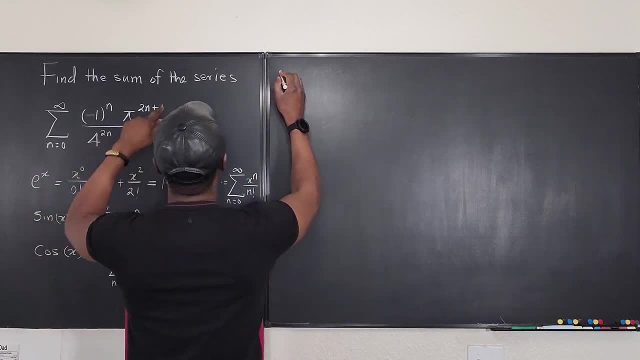 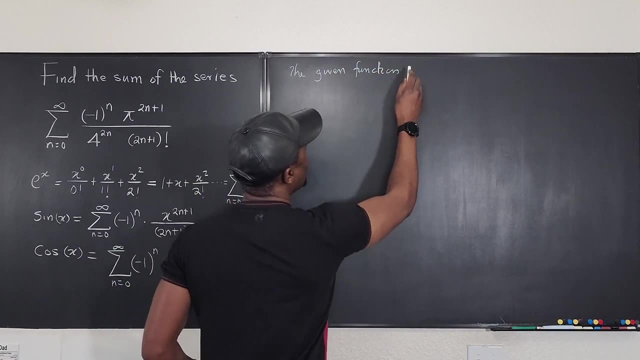 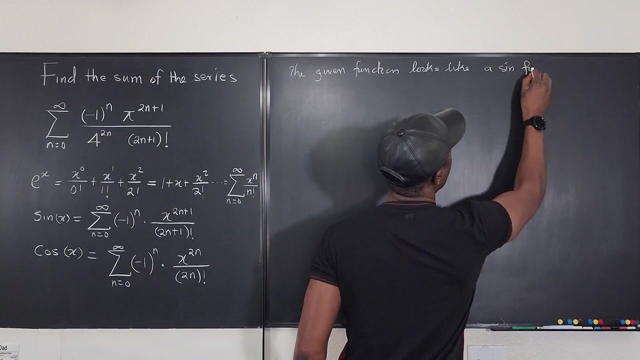 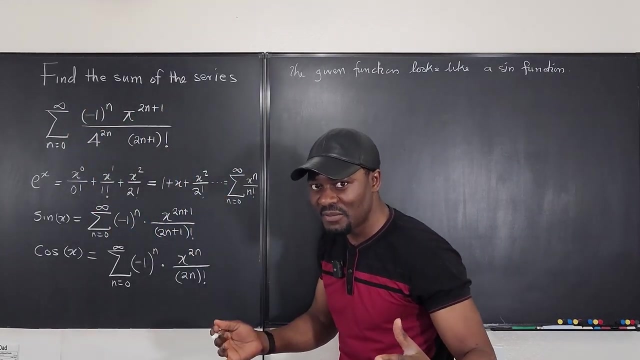 so let's say we're going to say that the given function looks like a sine function, so we know that signed something is equal to this. we just need to know what that something is. so let's look at the standard things that we always get in the sine function. 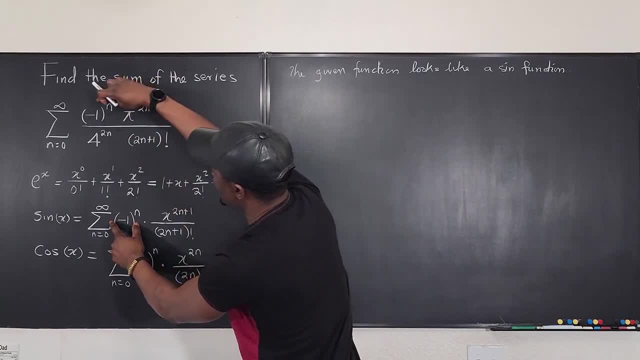 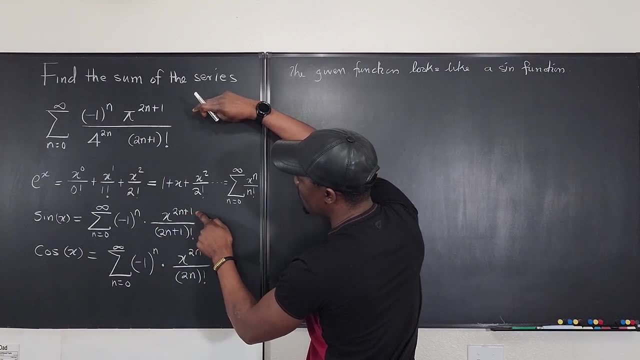 we know it's gonna have this. does it have it? yes, we know it's gonna have this. does it have it? yes, we know it's gonna have something raised to power, to n plus-one. yes, but this guy is just hanging out there. there's a problem with. 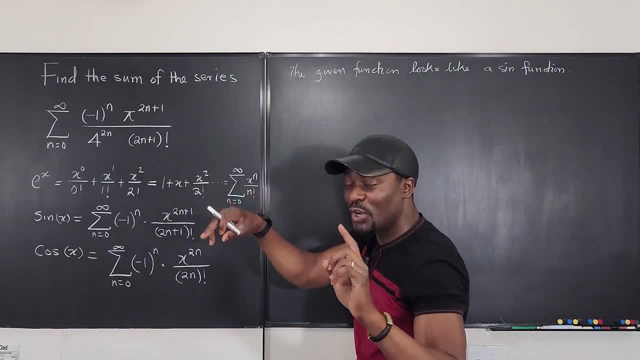 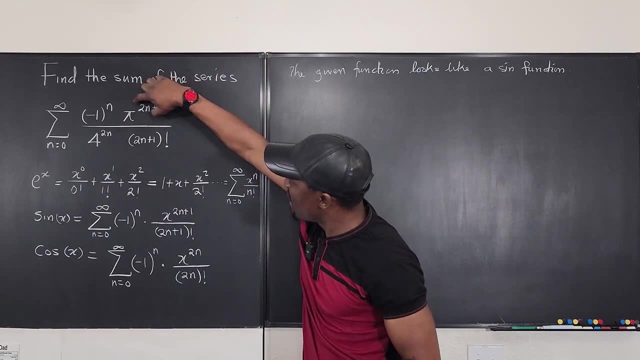 this guy? what should we do with him? ok, now I'm gonna show you that everything in your sine function has to be raised. if it is raised to an exponent, this has to be raised to 2n plus 1, and this must be raised to 2n plus 1. 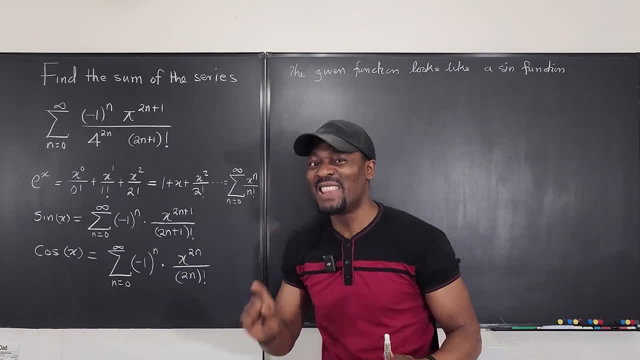 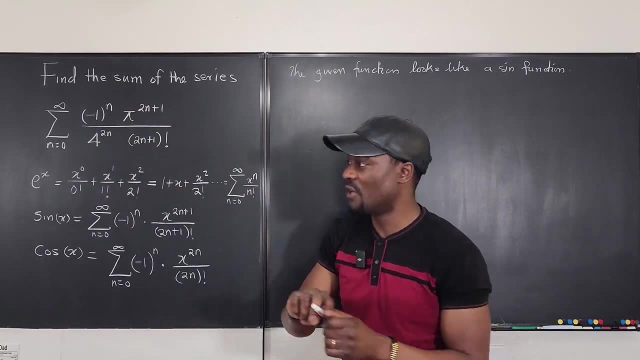 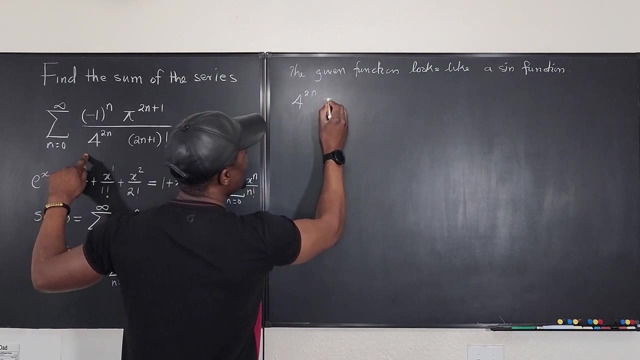 n plus one for you to be able to do any manipulation with it. and that's what we're going to do. we're going to change this to something four to the two n plus one and then adjust it to keep the value. so watch, we know that four to the two n can be written as four to the two n times four. 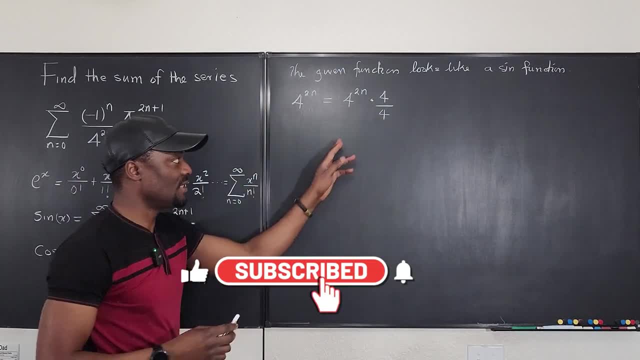 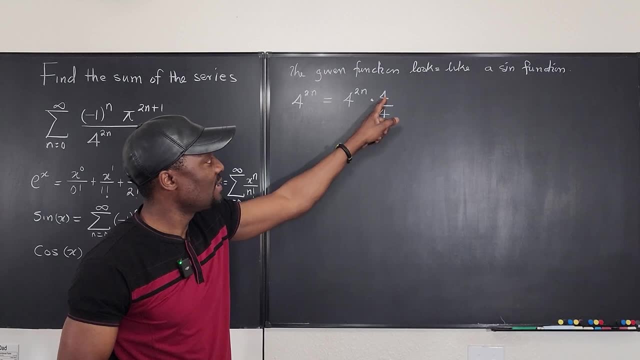 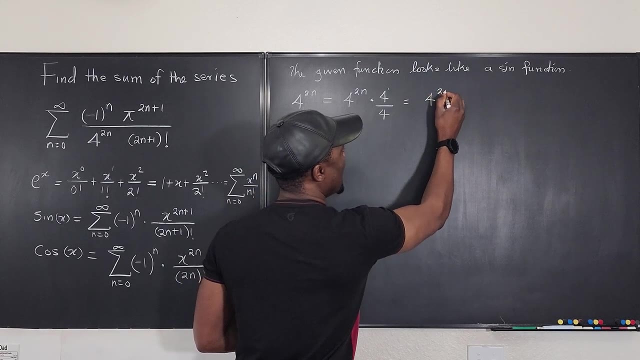 divided by four, see, this doesn't change anything. so four to the two n plus one is the same thing as this. but if i multiply this four by this four- see, this is four to the power one. this is gonna become four to the two n plus one. but now 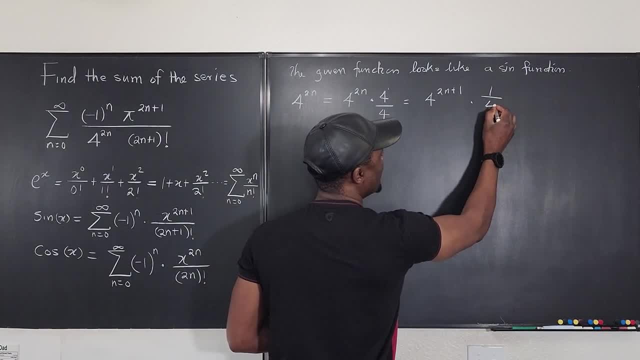 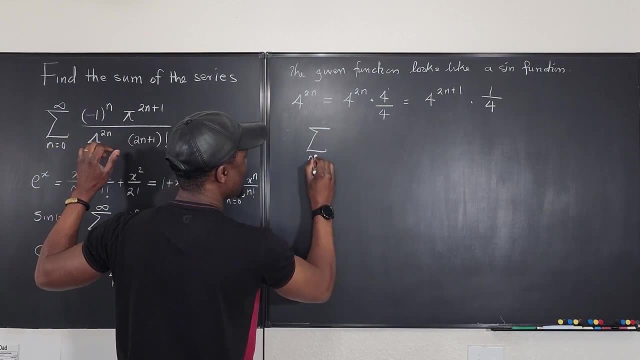 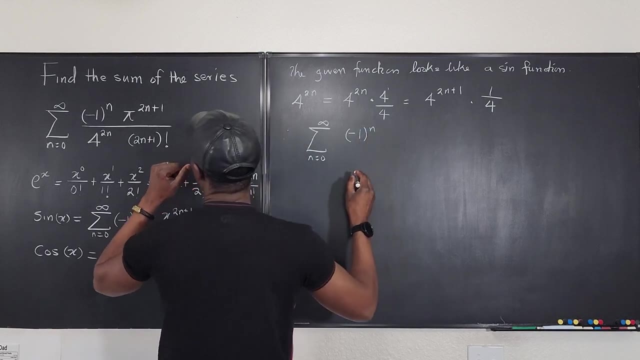 i am dividing it by four. okay, multiplied by one over four. so this expression, therefore this sum from n, equals 0 to infinity of. let's write negative: 1 to the n. divided by this is all divided by 4 to the 2n. 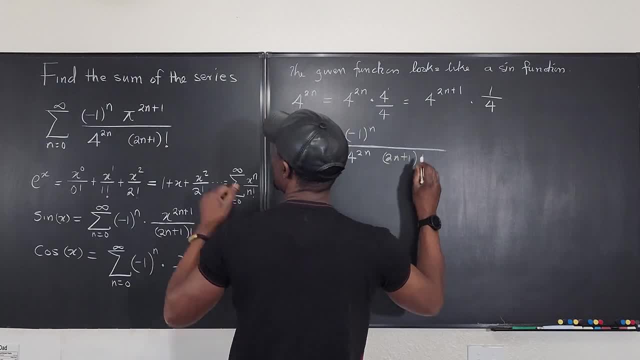 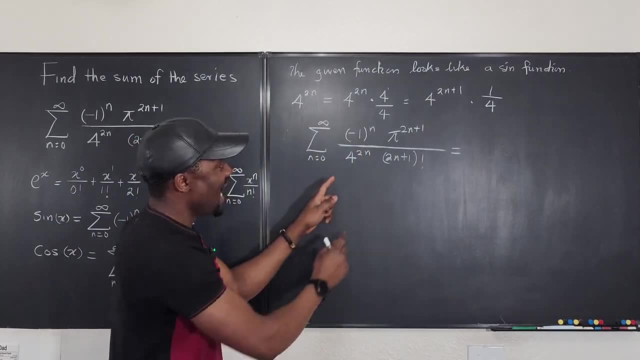 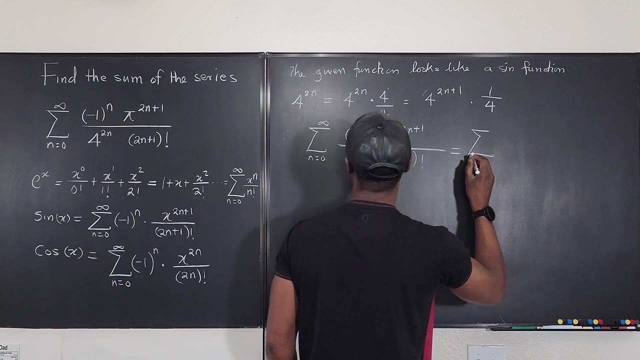 And then we have 2n plus 1. factorial pi to the 2n plus 1 is the same thing as now. I have rewritten this expression to look like this. So this is going to be the same thing as the sum from n equals 0 to infinity, of negative 1 to the n. 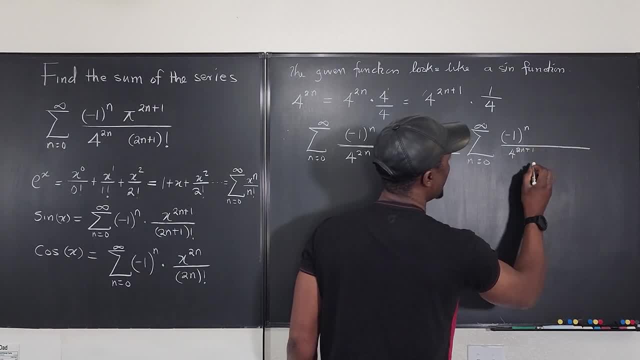 4 to the 2n plus 1 divided by 4.. Oh, I can bring the 1 over 4 all the way here. Let's put it here: Divided by 4 times 2n plus 1. factorial. 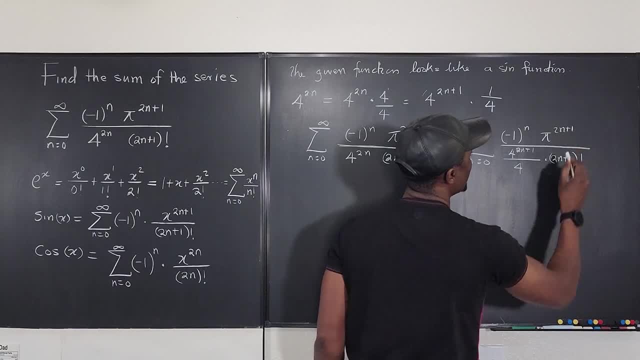 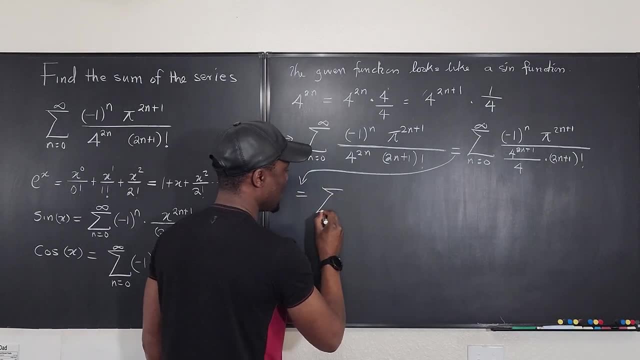 And on top I have pi to the 2n plus 1.. So this is equal to. This is equal to the sum. I think we're done by the end now. n equals 0 to infinity and I have negative 1 to the n. 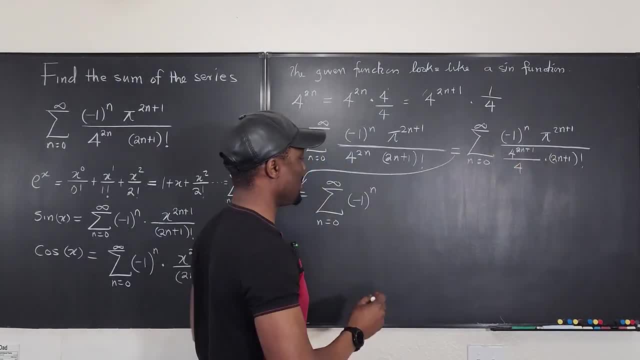 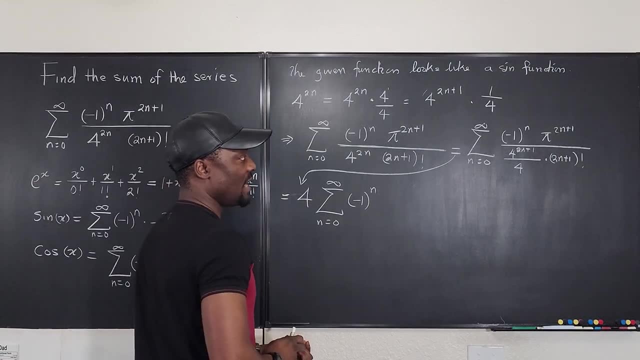 And if this joins this guy, this flips, it becomes a big giant 4, which I can actually write in the back here. since it's a number, It's not included. Okay, giant 4.. And here this goes here.